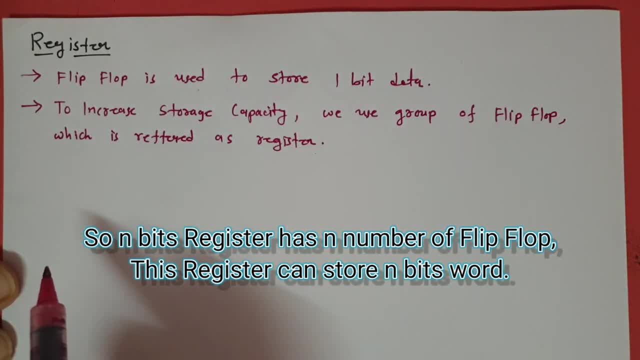 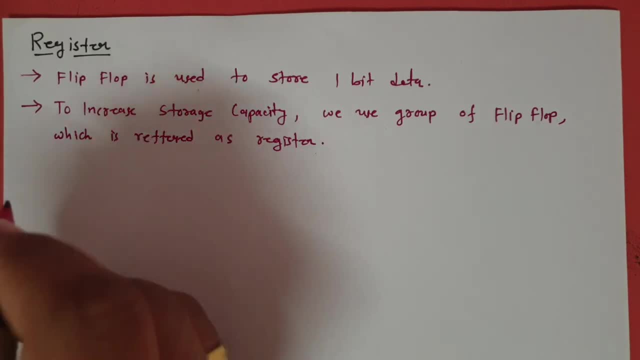 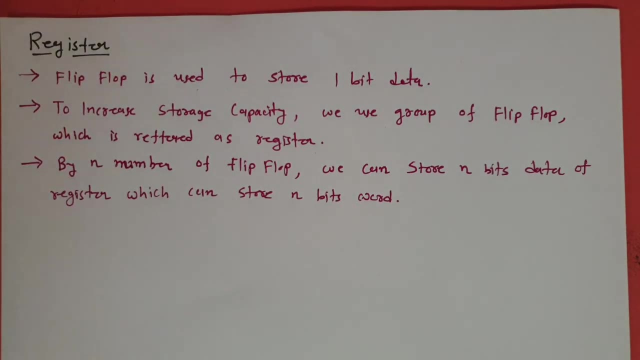 Then by that n number of flip flops we can store n bits word by using single register. So see, flip flop can store one bit data, but by using groups of flip flop we can make a register which can store more than one bit data. So let us have one example. 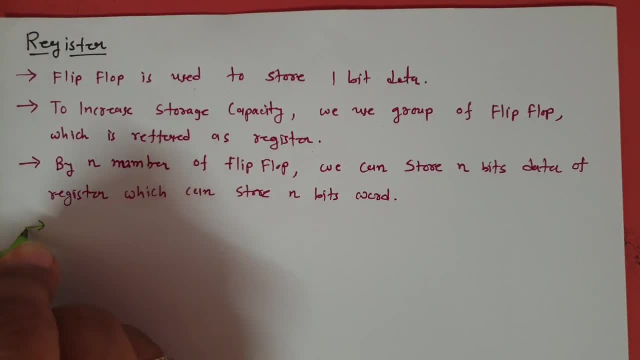 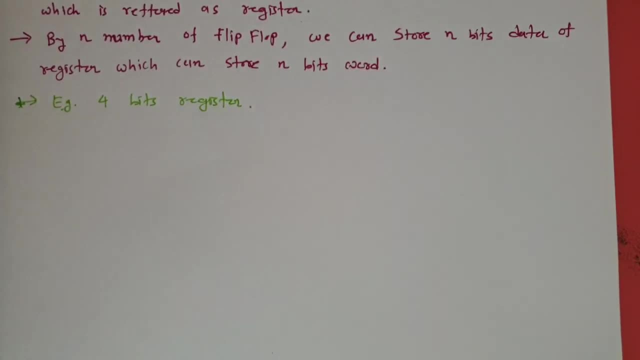 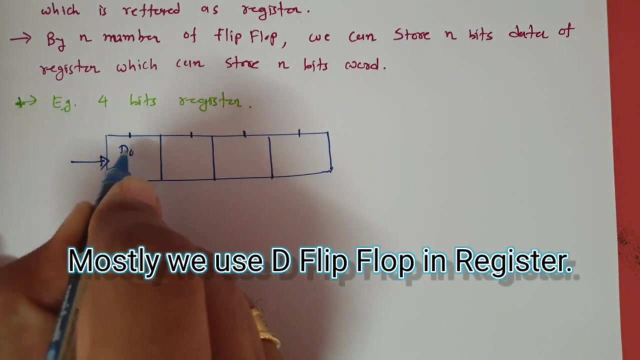 Where we have 4 bit register. Now in this 4 bit register we will be using 4 flip flop connection And in this 4 flip flop here we are giving clock and usually we use D flip flop. So let us say this is D0, D1, D2 and D3 terminal. 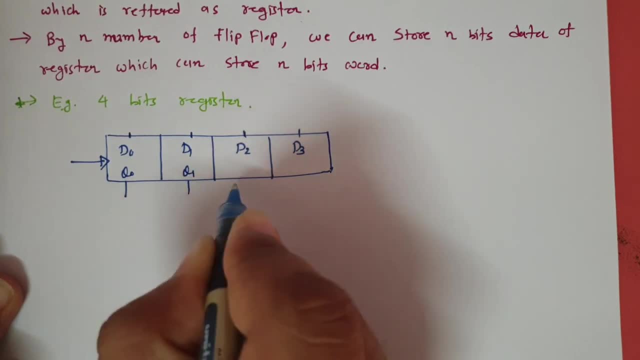 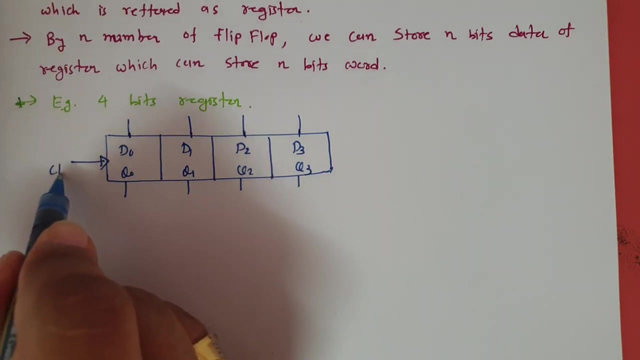 And here we have output that is Q0, Q1, Q2 and Q3.. So here we can store 4 bits data and here this is what our clock signal and this D flip flop can store: 4 bits. Right, If you see the working of the flip flop, then it will store data. 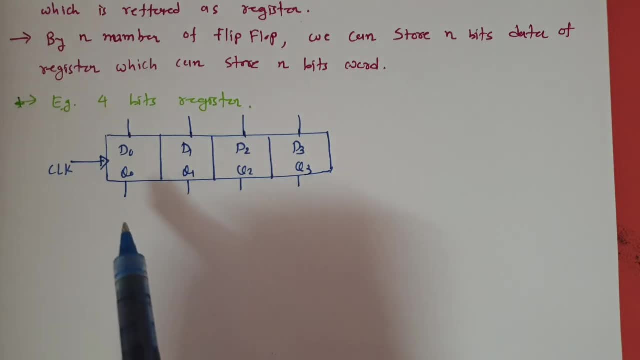 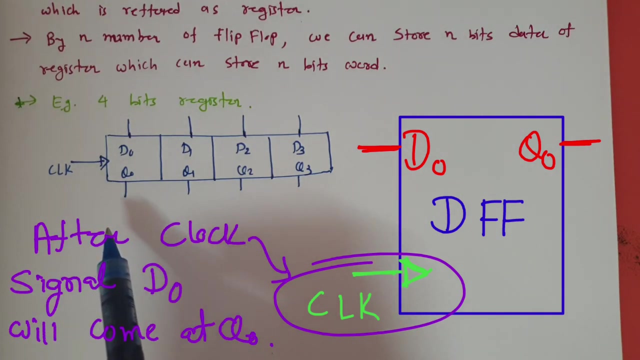 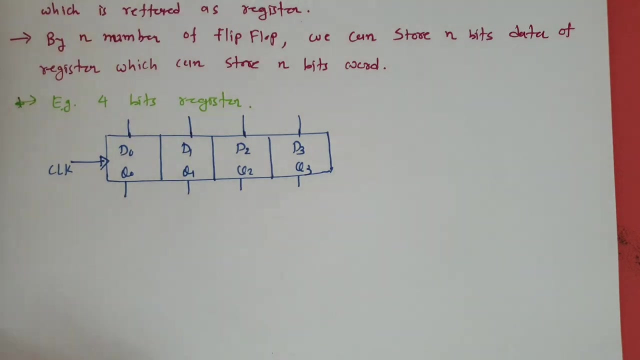 Then it will store data When clocking in clock is given. so for example, if D0, that is our input, so that input will get store and that will appearing at output side when clock is given. but problem is it cannot hold data for longer period. so to understand that, I'll give you one situation. for example, if I say: 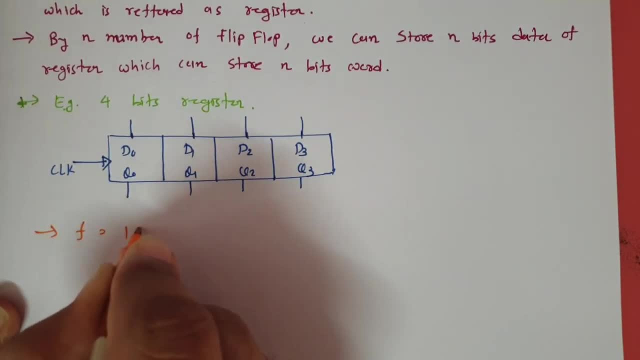 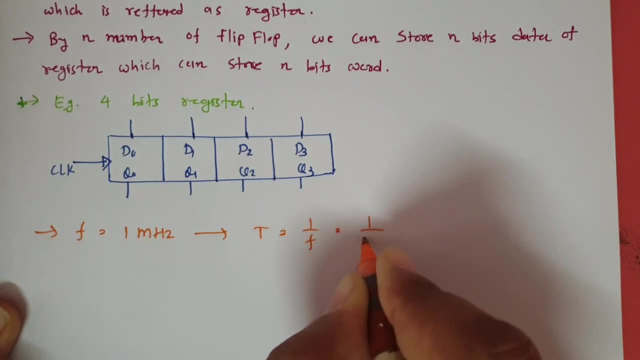 we have frequency f, that is 1 megahertz, then time period for the signal, that is 1 by f, so 1 divided by 1 megahertz, so that is 1 microsecond, right? so if you observe the signal of 1 microsecond, 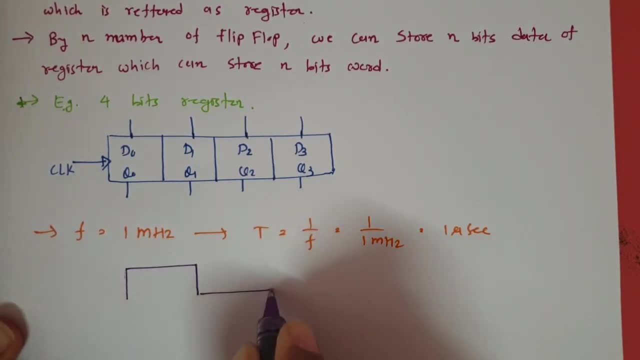 then if you observe this clock of 1 microsecond, then you see here for this time period f that There is 1 microsecond, and if this is active high clock, then for this much time period only it will be holding data. This complete time period is 1 microsecond and this is what the time period which is 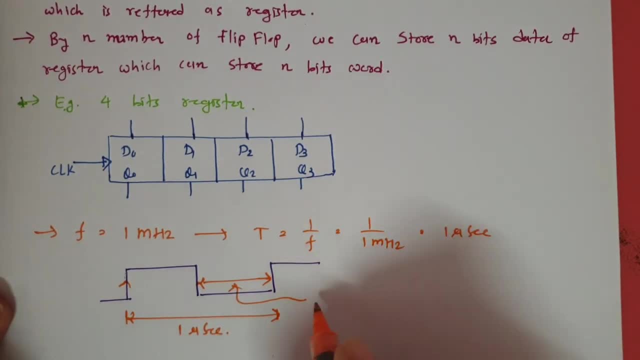 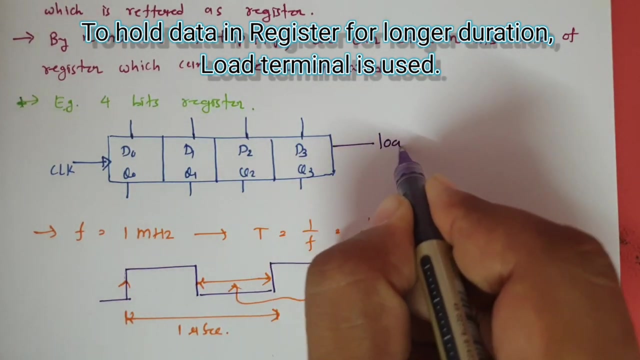 what holding storage data. So here we have very less time period for which this data that will get stored in this register. So there are some additional functionality which we added to hold data for longer duration. So there is one more additional facility which we add, that is load. 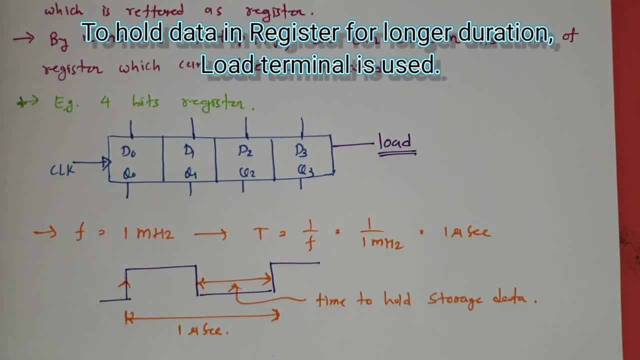 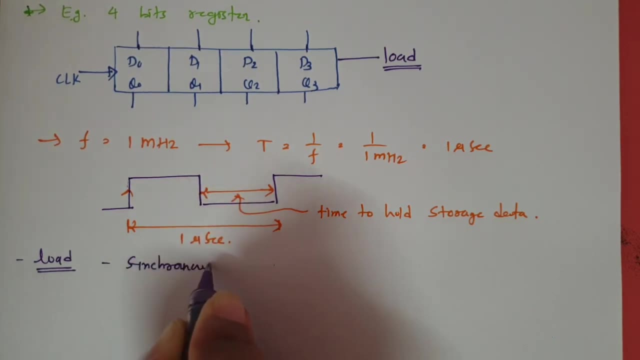 So by this load terminal, we can hold data. Now you see how load is holding data for longer period. So there are basically two types of load which is there with us. One is synchronous load And second is asynchronous load. Now, when we talk about synchronous load, 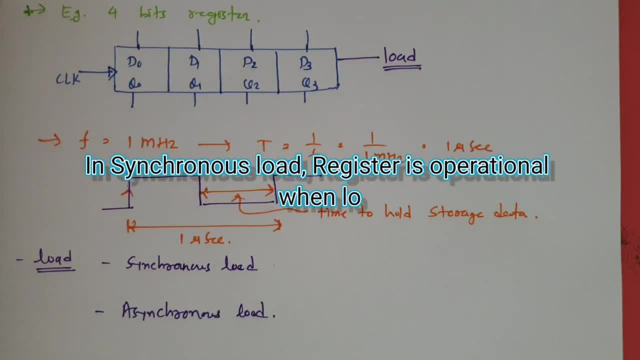 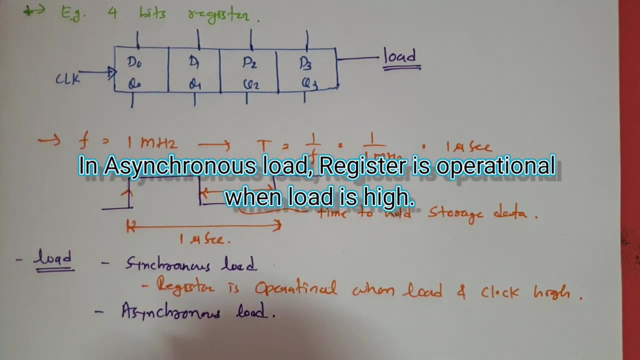 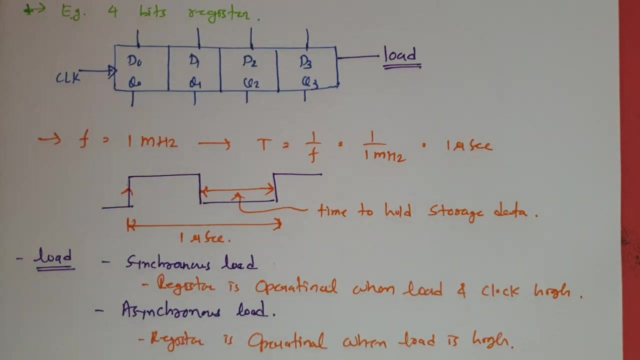 So in synchronous load you will be finding this register is operational during load and clock- both are high. And in asynchronous load, register is operational when load is high. Now see what is the meaning of this. See previously. if you observe, if clock frequency is 1 megahertz, then the storage data of this 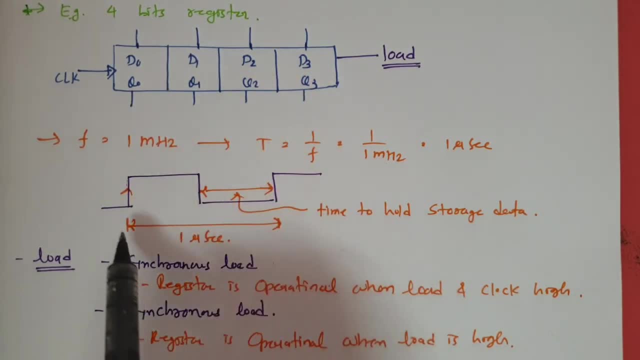 register that will be there at output side for this period only right where for this time period, only this register will hold data. So if you want to hold data for a longer duration, Then we are adding one more register. That is load. Now see what happens by load. 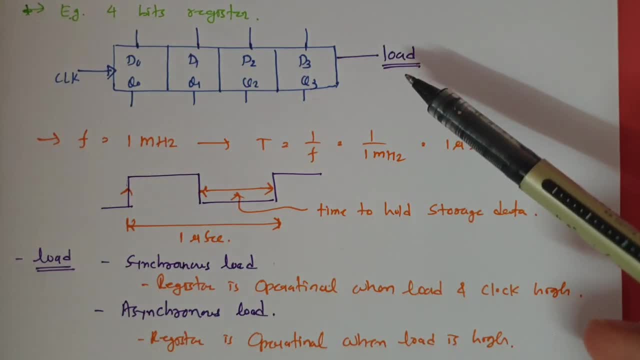 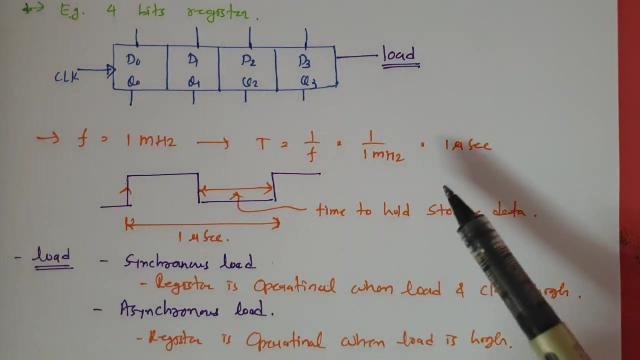 Because of load. when you keep load high, at that time register is operational Like see: for synchronous load, load and clock should be high and for asynchronous load, load should be high. So what happens is like when load is high, at that time only we can change data of register. 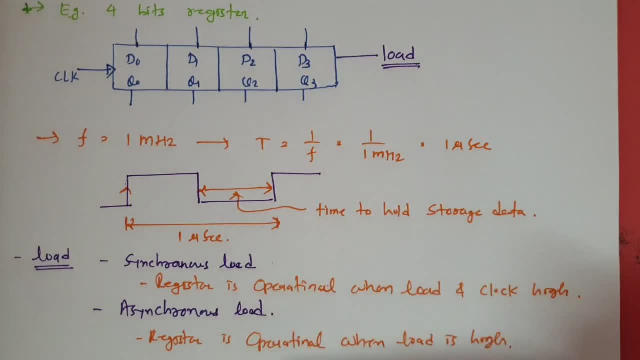 So, for example, if you have asynchronous load, In that case you can change data of this register when this load is high. If this load is low, in that case one cannot change data of this register, While in synchronous load we should be giving clock signal as well, as load should be high. 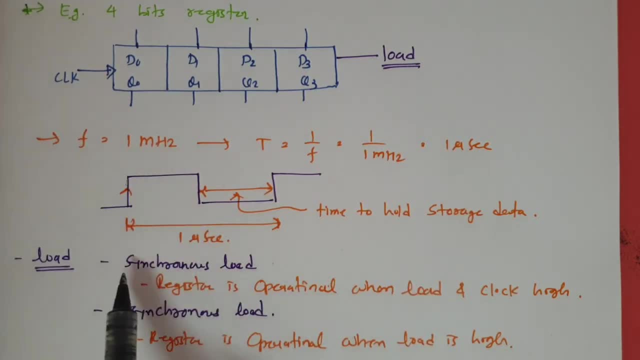 So if both are active, in that case synchronous register will be operational, means we can store another data in this register Right. So we got additional facility which we added in register to hold data for longer time period. So when load is low, at that time there will be no change at output side and it will store. 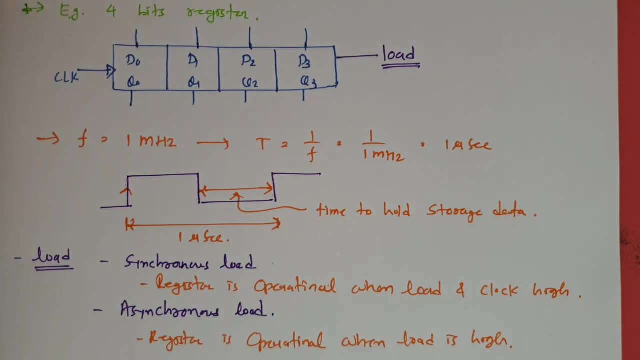 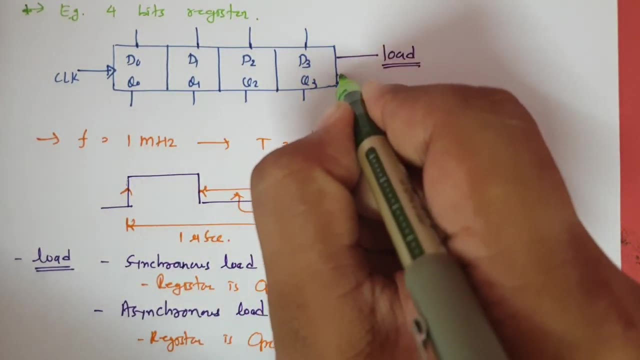 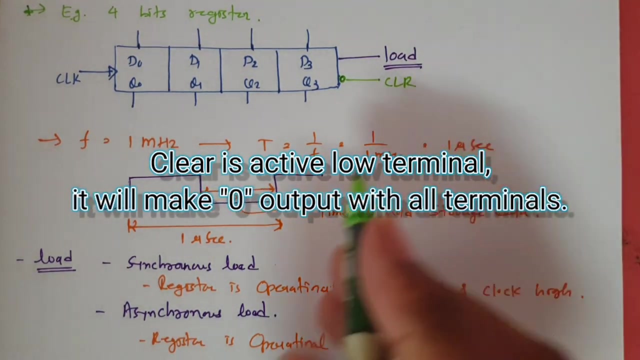 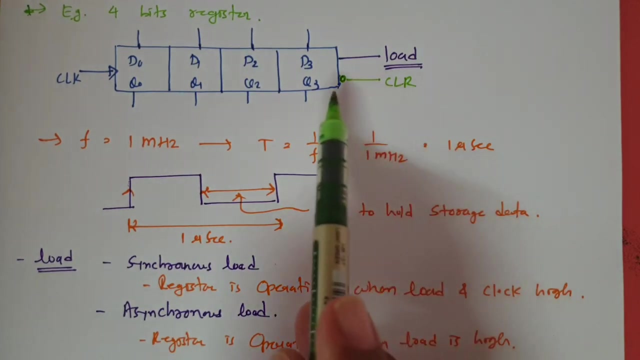 previous data. Now one more thing that one should know, that is to have clear operation. So if you have connected clear signal over here, Then this clear signal that will clear data of all this register right. So after clear means, active low signal at this terminal. all four output: q0, q1, q2, q3, that 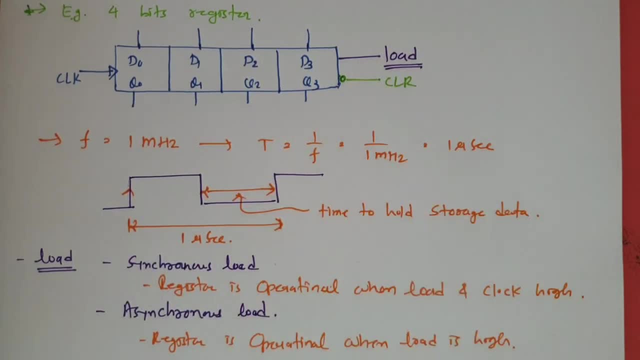 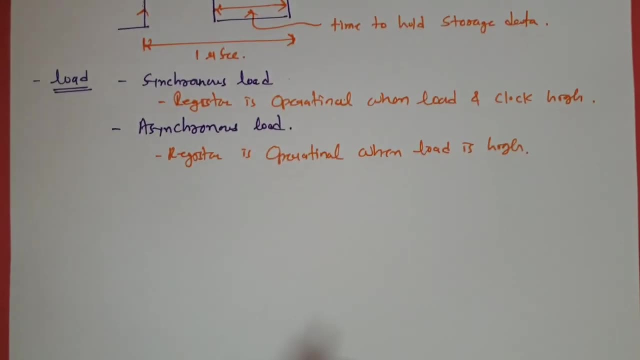 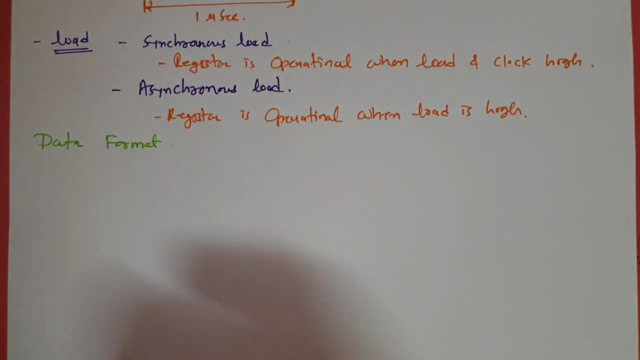 will get zero. So this is even one more additional feature which is there with register. Now let us discuss some important points, which is data format. So in register there are basically two types of data. One is serial data format and second is parallel data format. 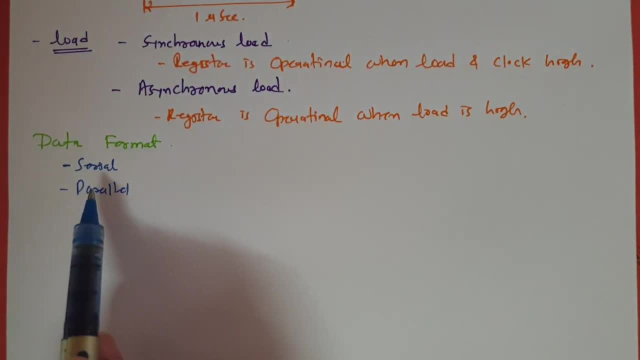 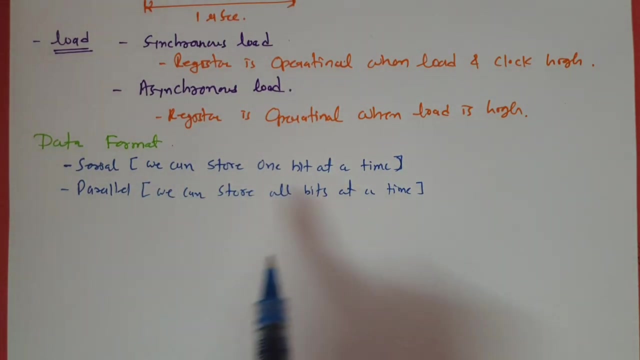 See, in serial data format we store one bit at a time in register and in parallel data format we store data parallelly in register. So basically there are two types of data format, which is there with register. In serial data format we store one bit at a time and in parallel data format we store 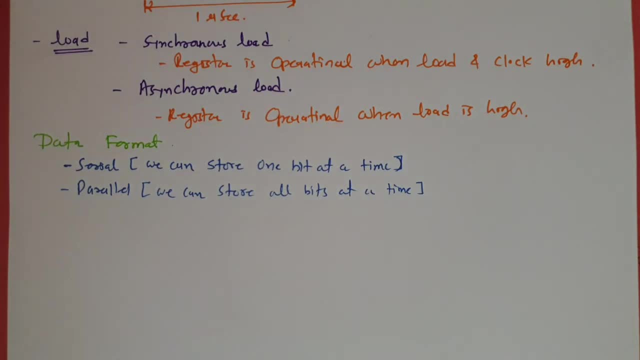 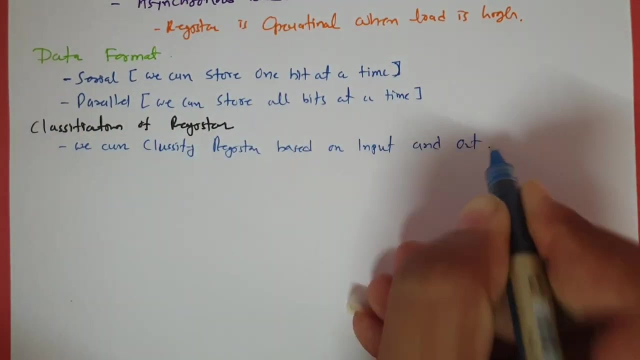 all bits at a time. Now I'll explain you all those things in classification with more detail. So let us classified register So we can do classification of register based on input and output. So when you want to classify register based on inputs and output, 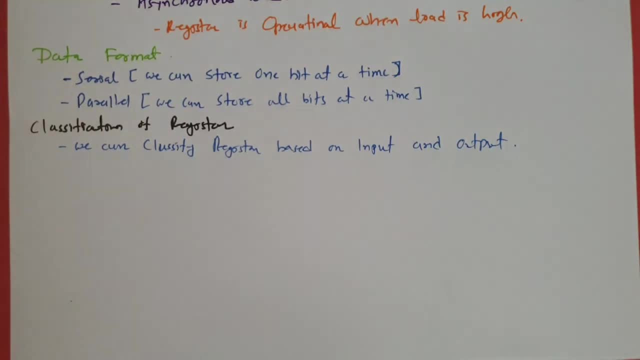 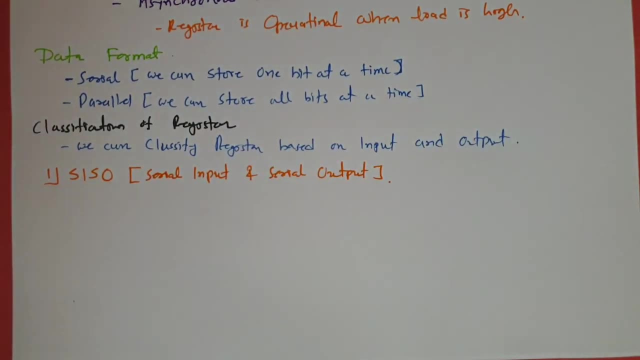 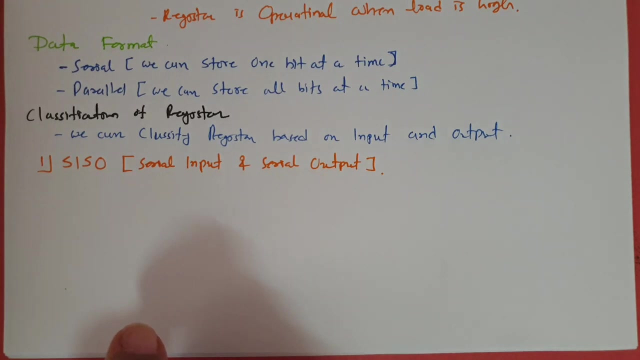 Then you should know that register is in serial data format. So when you want to classify register based on inputs and output, Then see first type of register, that is, serial input, serial output. Now see in serial input, serial output, we enter data serially in register and we take data output serially from register. 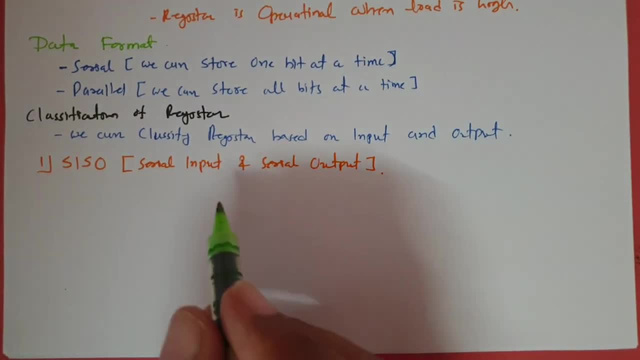 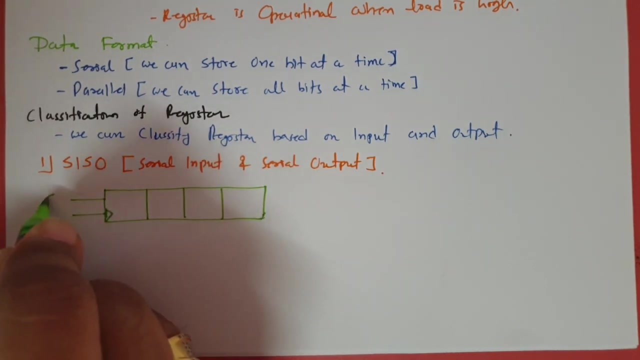 Right. so in SISO means serial input, serial output. types of register: we enter data serially. So you see, if I have register over here, here we provide a clock signal. So here serial input is there and here we have serial output, right. 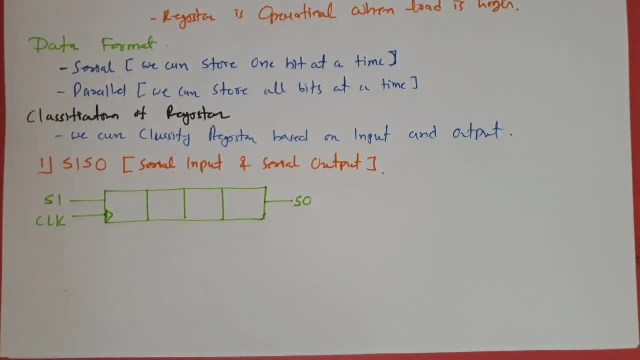 And see these four boxes. those are flip-flop inside. So In serial input, serial output types of register, we enter data serially and we take data at output side in serial manner, right? So one bit that we can enter at a time and one bit that we can take it at output. 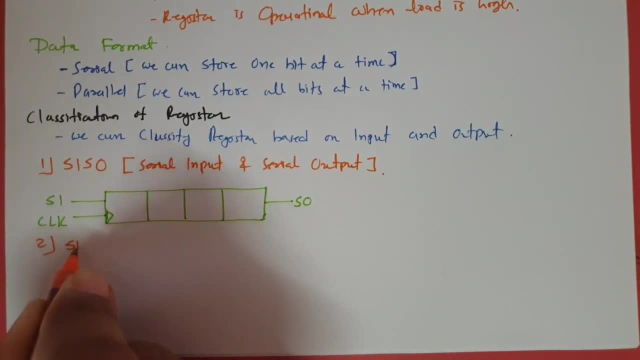 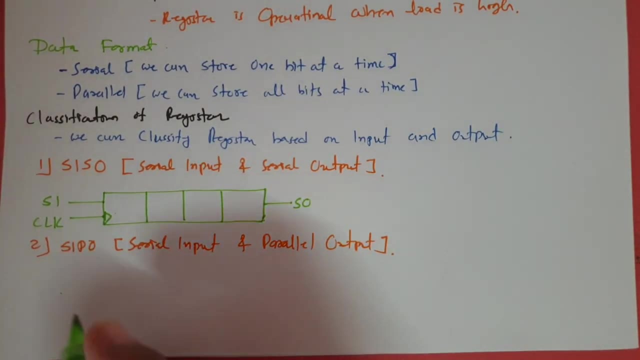 Now second type, that is serial input, parallel output type of shift register. So in serial input, parallel output type shift register you will be finding We enter data serially. so you see, these are four flip-flops which is there inside. Here we provide a clock input that is given as serial input, but output that will be parallel output. you see. 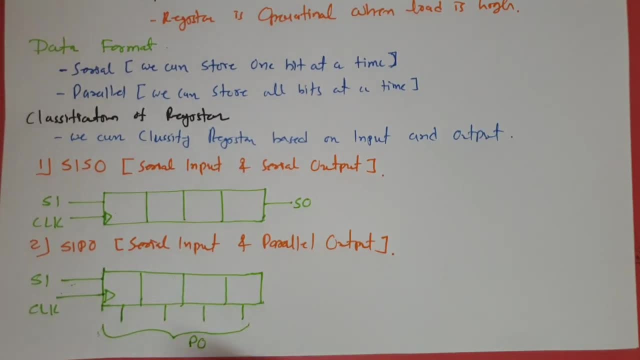 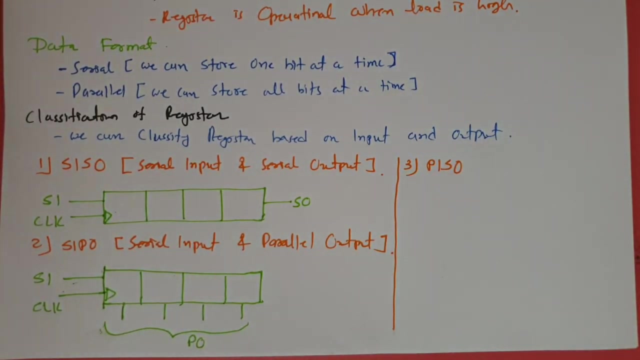 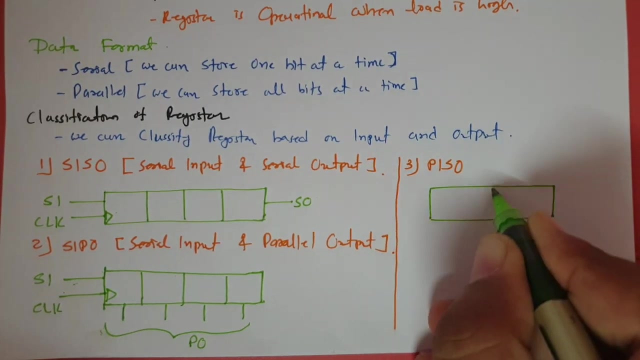 So this is my parallel output. that is what serial input, parallel output, type of shift register. right Third is parallel input, serial output. Third is parallel input, serial output. So in parallel input, serial output you will be finding we give input parallelly. so if you have flip-flops, you see I am connecting four flip-flops here- we provide a clock signal. input is given parallelly, you see. 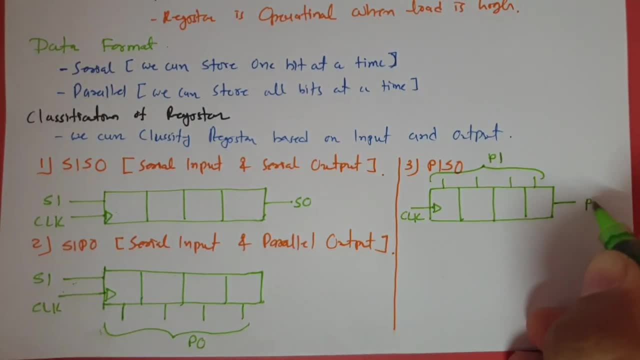 So we can say: parallel input, but output that we take as serial output, Right, so output that we take as serial output. so this is what? serial input, sorry, parallel input, serial output. Now fourth category, that is parallel input, parallel output, where we give parallel input.